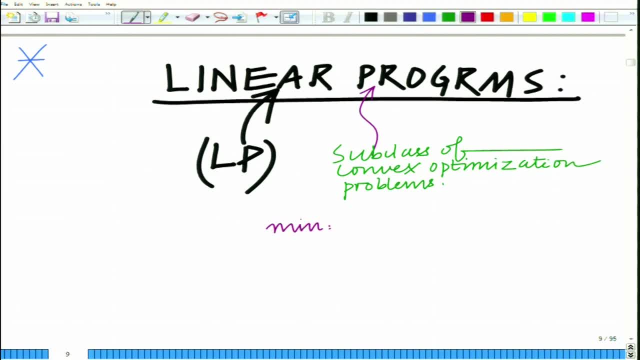 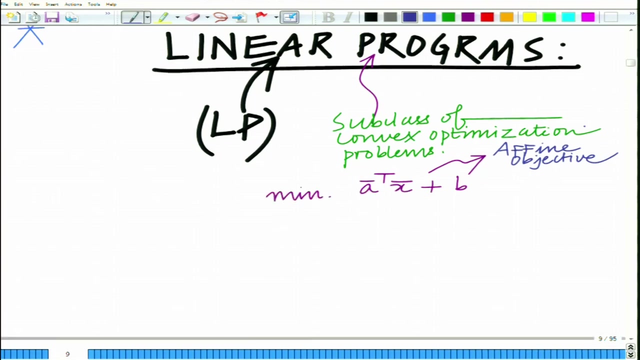 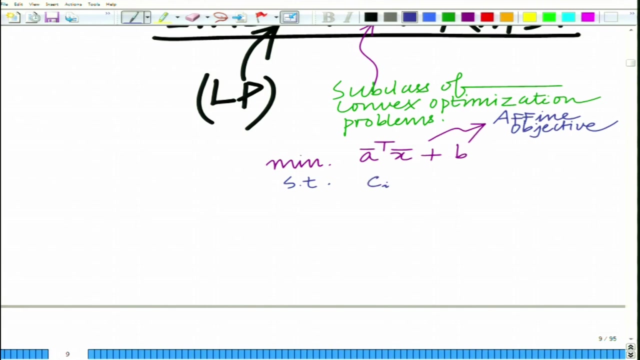 be expressed as follows. that is, remember, any convex optimization, any optimization problem has an objective. So let us minimize a bar transpose x bar plus b, which basically has a linear objective or an affine, an affine objective function subject to the constraints, which are also affine, that is, c bar transpose c i bar transpose x bar less than or equal to. 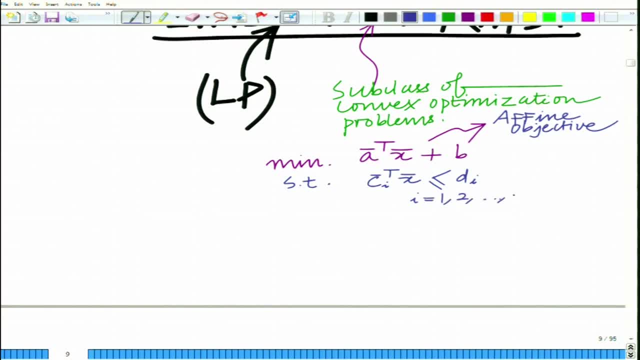 d, i for i equals 1, 2 up to l and equality constraints, which have to be affine in any case for a convex optimization problem, as we have seen in the previous module, that is c tilde j transpose. So x bar equals d, tilde j for j equals 1, 2 up to m. all right, So basically the constraints. 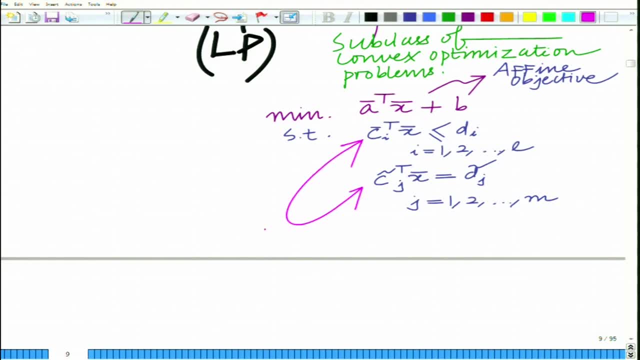 the equality as well as the inequality constraints. all right, So all affine, that is, it has affine equality and slash x bar equal to d, tilde j for j equals 1, 2 up to m, So it represents an này or or. 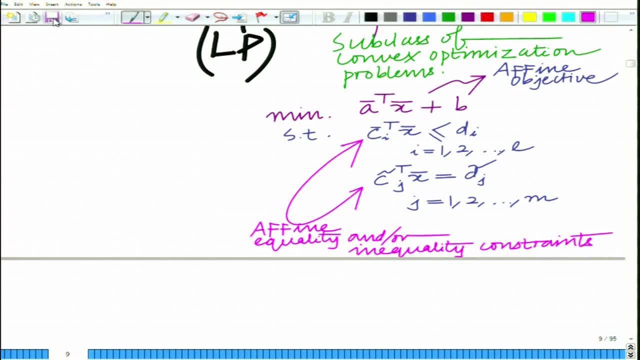 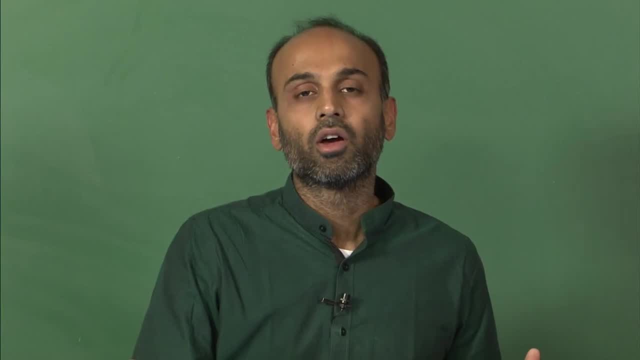 It is the binary with sign imposed in this compound into nurse. So here it will be called a lineartem snatch, where this also it will be known as Secure constraint. that is some linear example So we are able to find out its Sanders. 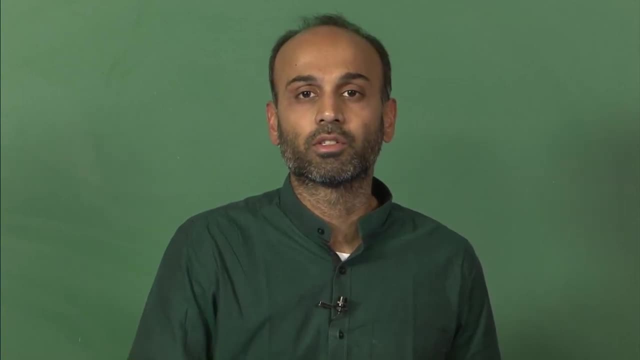 S Right, So it is not certain. There are 여�, n, n and docs. All right saben, there isn't a winner right now and there is one more. therefore, this is a special class of convex optimization problem, So a linear program. 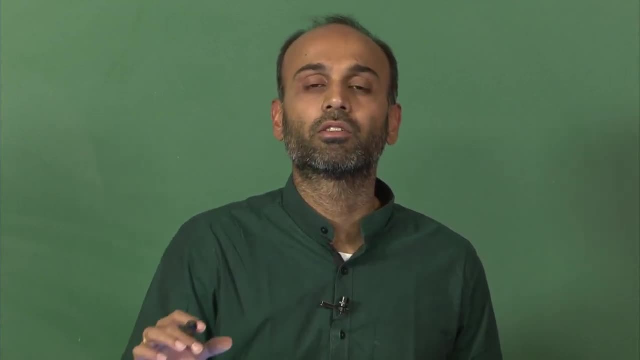 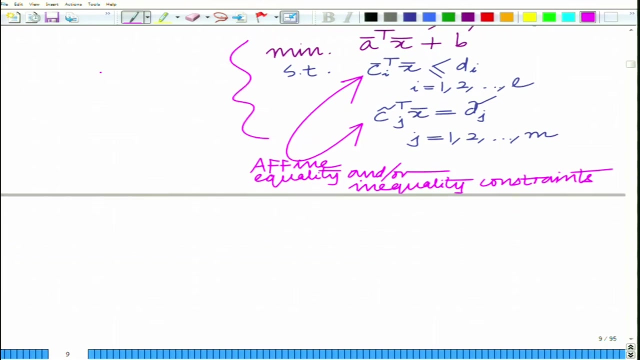 is a special, is a subclass of convex optimization problems in which the objective function as well as the constraints, equality as well as inequality. constraints are all affine in nature And you can say: this is so. this is basically your linear program. And well, you can say: this is the simplest, because everything is. 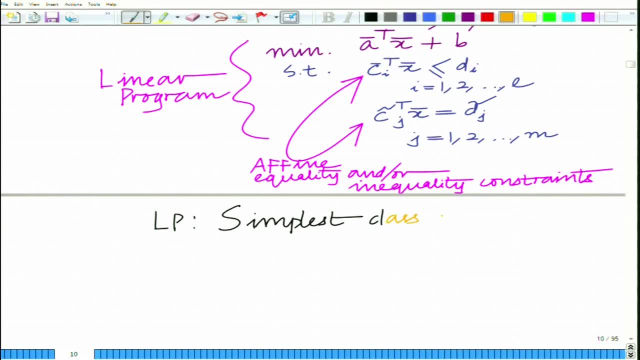 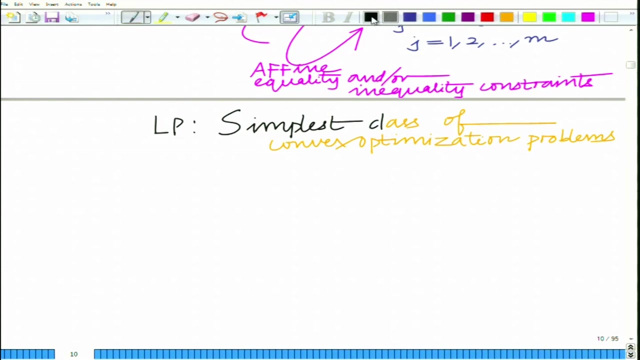 affine. this is the simplest, simplest class or category of linear program. So this is the category of convex optimization, of convex optimization problems. Now, just for convenience, I can write this in matrix form. So I can represent the L? p in matrix form as follows: 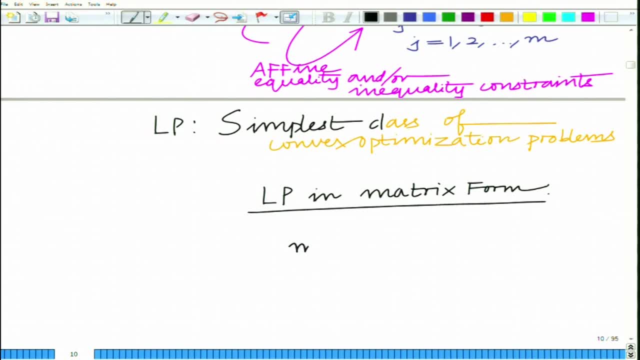 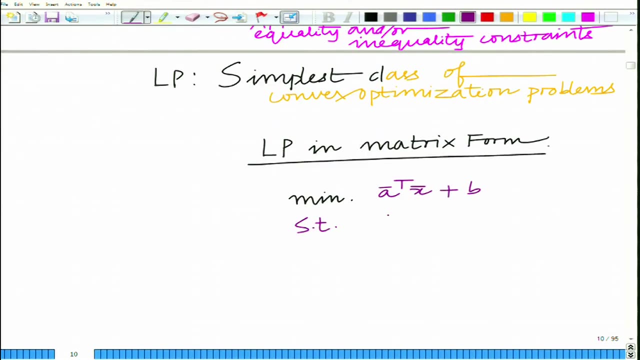 it is not very difficult. So I have minimized the objective, which is: a bar transpose x bar plus b, subject to the constraints. Now, constraints, I can represent them as a matrix, So I can write this as: c 1 bar transpose c. 2 bar transpose c. l bar transpose x bar plus b, So I can write this: 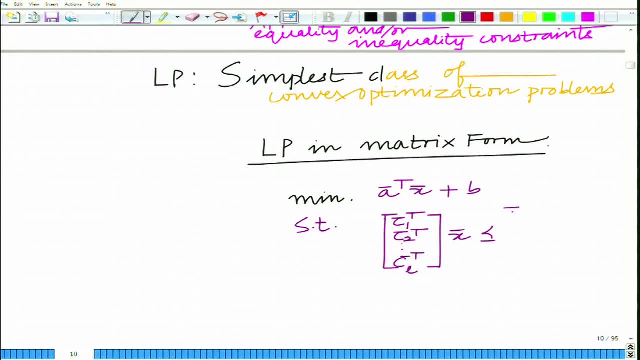 as c 1 bar. Now this is component wise, that is, each component of the vector on the left has to be less than each component of the vector on the right. So this is a component wise is also remember is also termed as component wise. 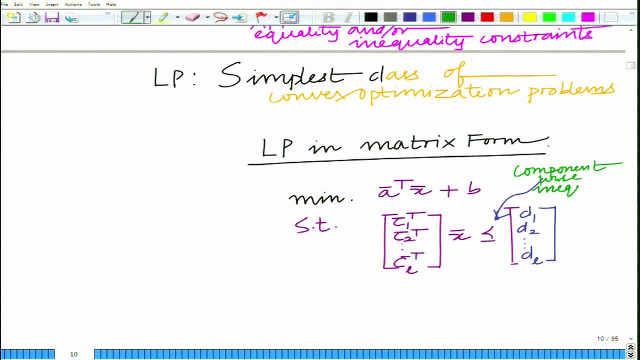 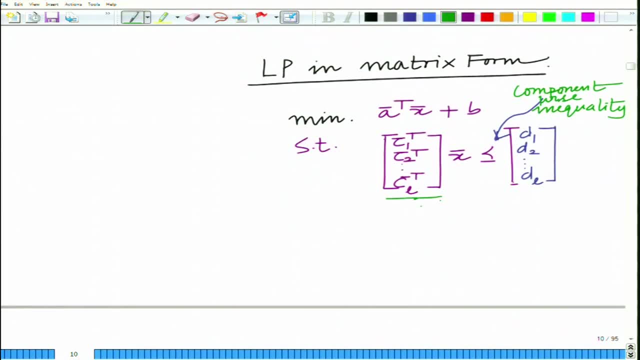 So this is the component wise, inequality. so I can write this now as your matrix c times x bar, component wise: less than this is your vector d bar. alright, So I can represent it in a compact form using matrices. similarly, the equality, mitochondrion constraints, I can. 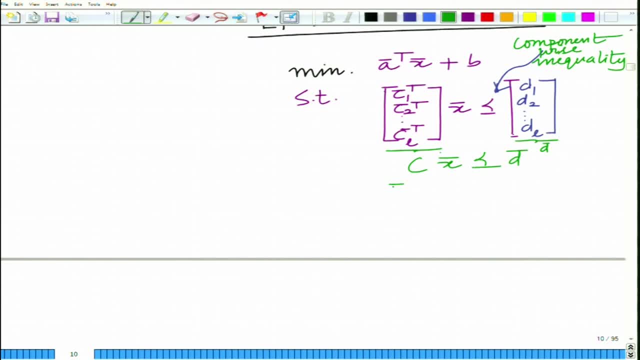 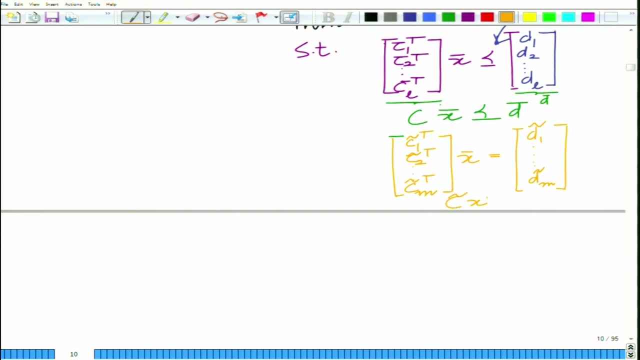 represent them As: C 1 tilde. transpose C 2 tilde. transpose C m tilde. C m tilde transpose times X bar equals C 1 tilde. up to D m tilde. So this becomes your C tilde. X bar equals D tilde and therefore: 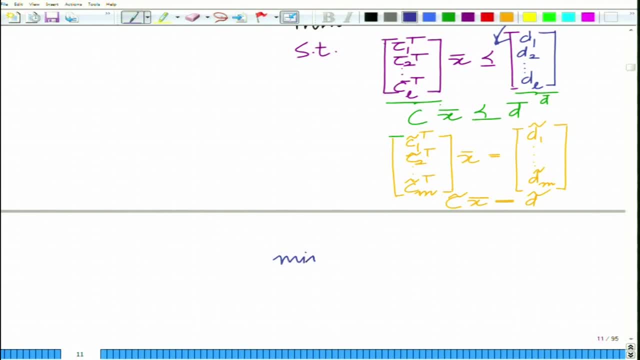 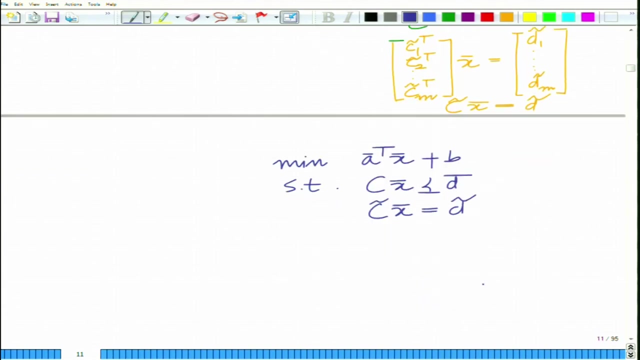 the compact. this can be written in compact form as follows: minimum: minimize A bar. transpose X bar plus B subject to C: C: X bar component wise less than D bar and C tilde. X bar equals D tilde. So this is a. you can say a compact form for a. this is the compact form for the linear. 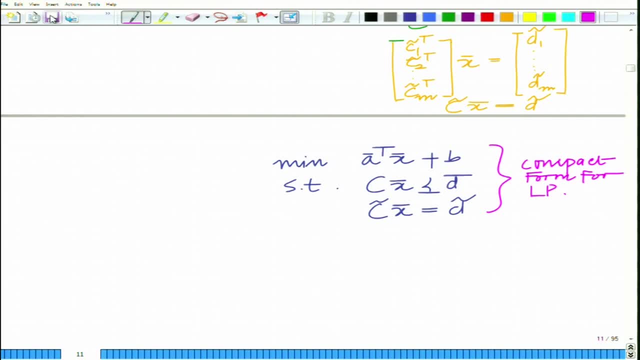 So this is basically expresses your linear program in a very compact form. in a compact form using vectors and matrices. Let us look at an example for this linear program- and we have already seen this before, that is, we have already introduced this before, that is. 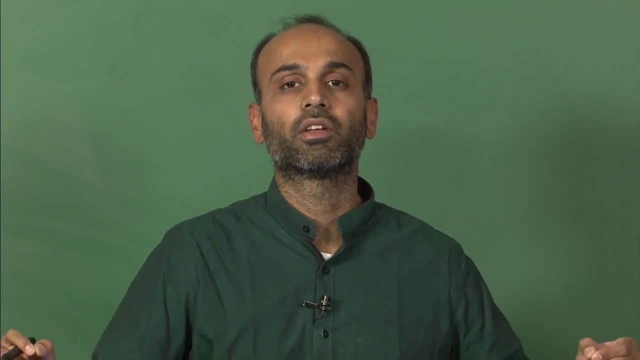 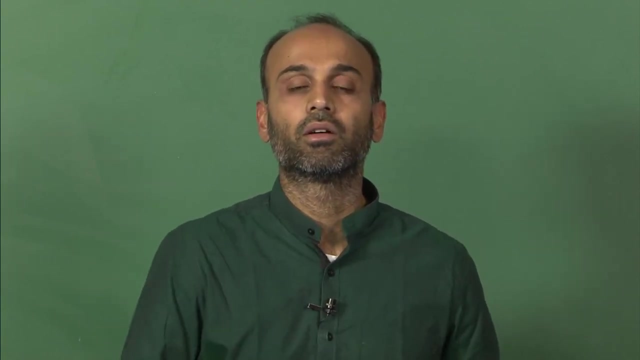 the example of base station cooperation, where there are several base stations in a cellular communication scenario. Where is the user at the edge of cell, At the edge of several cell, or the intersection or the region that can be served by several cells, all right, or can be served by several base stations. So the different base stations. 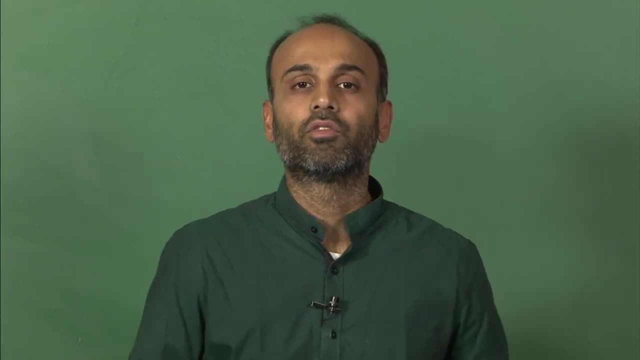 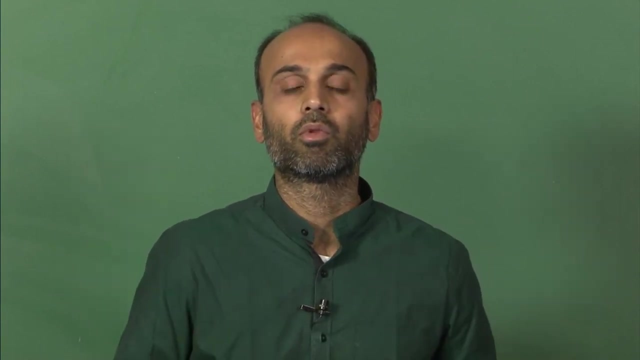 typically, when the user is at the edge of a cell or at the edge of cells, the user can be served by several base stations belonging to the different cells which are overlapping at that particular point, And so we consider a scenario in which this particular user is. 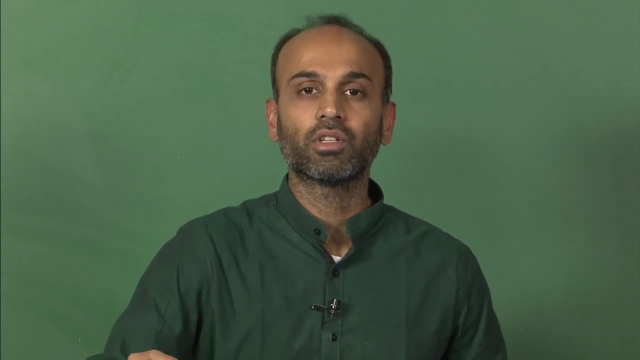 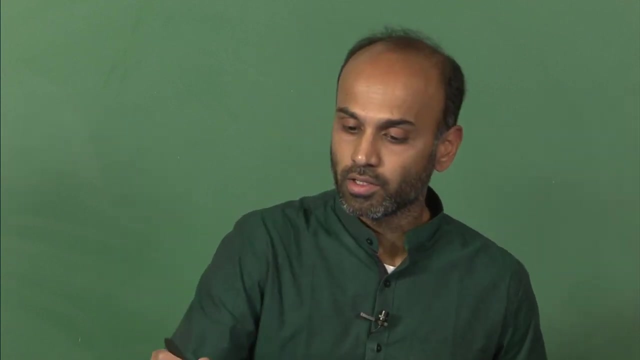 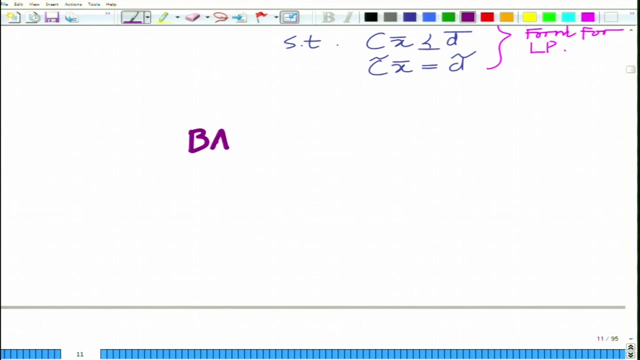 being served by several base stations or not just one: the single user. in fact, several users can be served, But when the by different base stations cooperating with each other, all right. So let us take a look at our example of base station cooperation or cooperative. 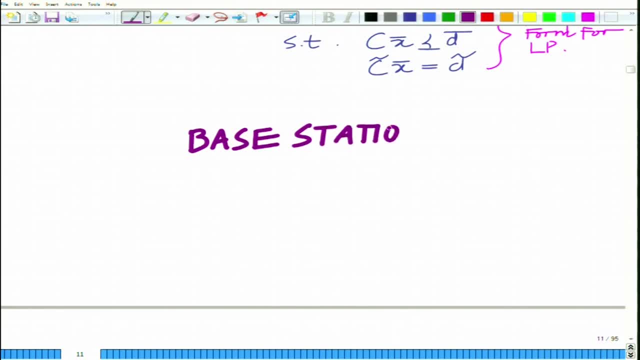 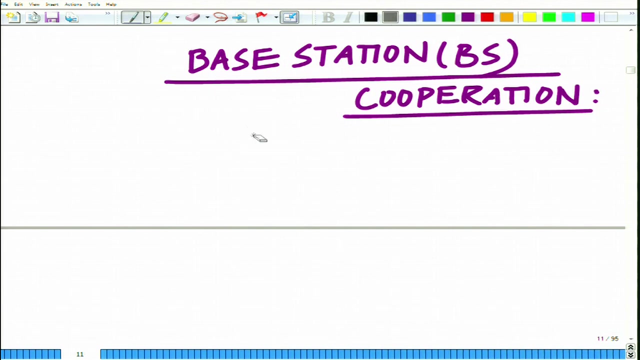 I have different users. The base stations are transmitting to the various users in a cooperative fashion. Normally, 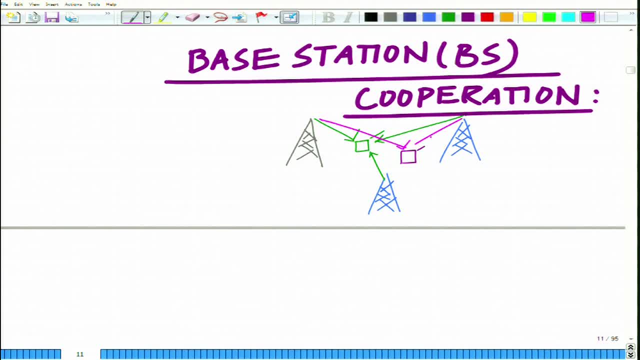 we have a single base station serving any particular user, but in this particular, this particular scenario, base stations can cooperate to serve the various users. thereby enhance the SNR, enhance the reliability of communication in a wireless communication. ции by enhance the SNR, enhance the reliability of communication in a wireless communication. 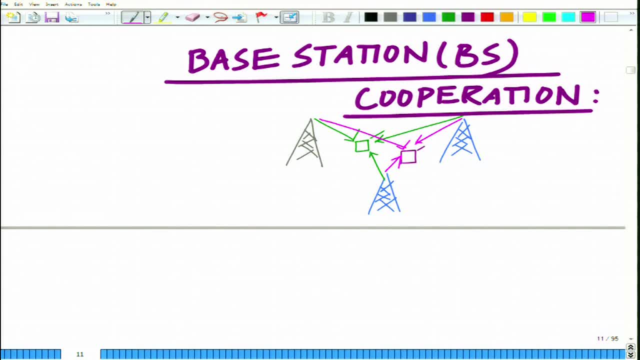 scenario in a wireless cellular communication scenario. So this is basically your base station. So we will consider a scenario in which we have K, So we have K base stations and M So K base stations are cooperating in this cooperatives cellular scenario. to 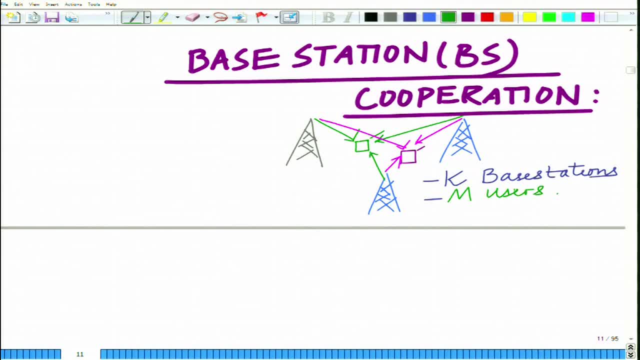 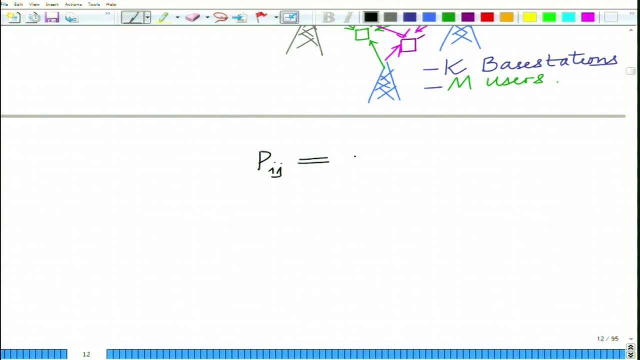 serve basically M users And in this scenario, like p i j, it would denote the power of power transfer, The Power Of transmitted by base station i to user j, And we will denote by h i j is the feeding channel coefficient. So magnitude h i j square equals g i j represents the power gain, the. 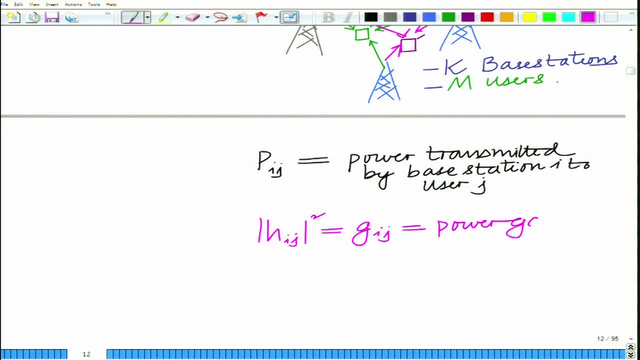 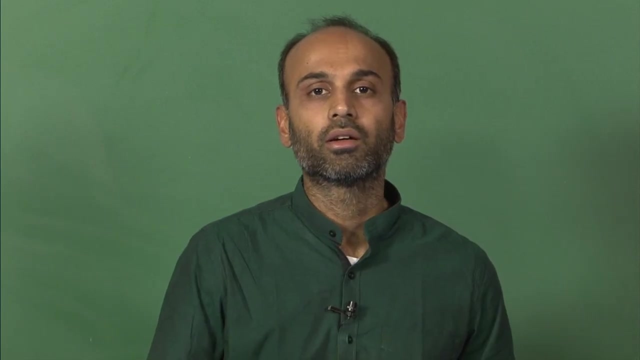 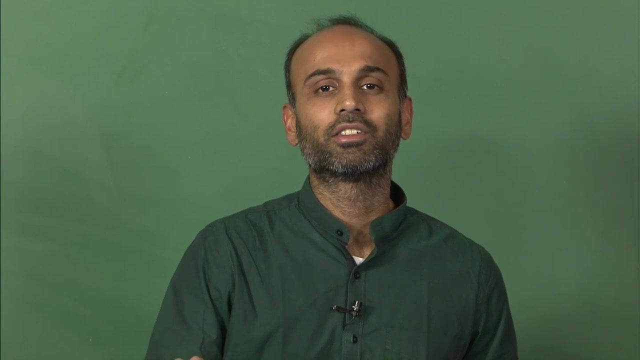 power gain between base station i, base station i and user j. So p i j denotes the power transmitted by base station i to user j and magnitude h i j is the feeding channel coefficient. magnitude h i j square, which is g i j, represents the 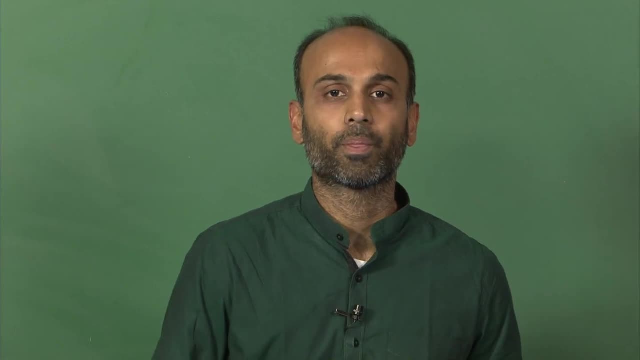 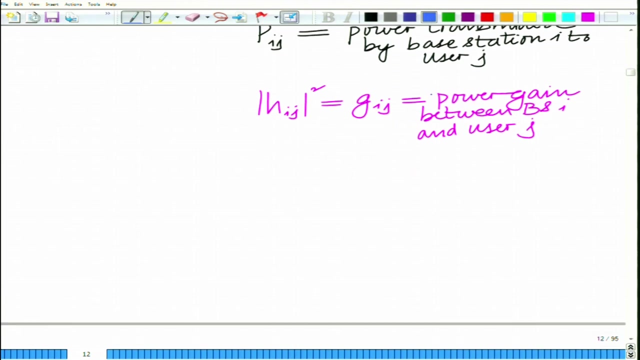 power, the gain from base station i to user j And therefore now, if you look at the power that is received by each user i, So the power that is received by each user i in this cooperative fashion is the power, some of the powers that 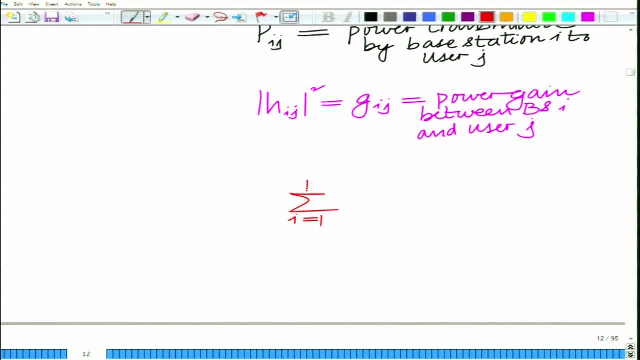 is transmitted by all the base stations. So I have i equals 1 to K, p, i 1, g, i 1, this, basically, is the power received at user 1.. This is the power received at. this is the power that. 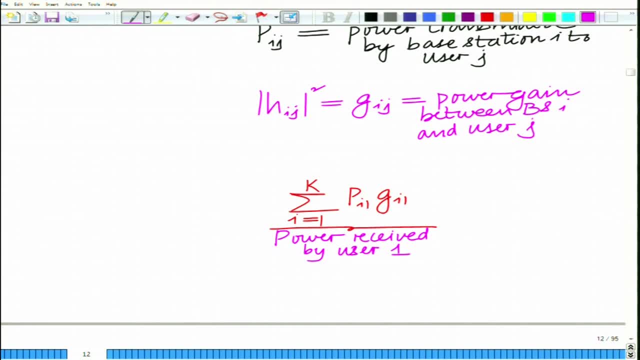 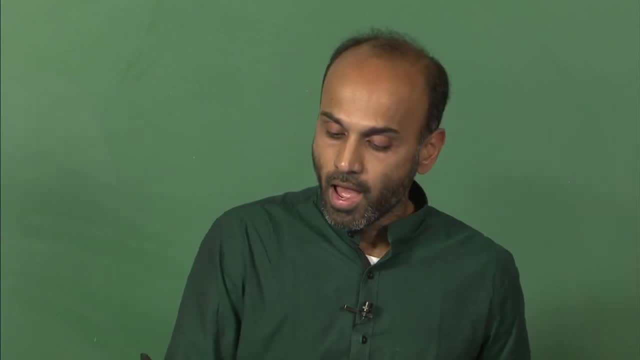 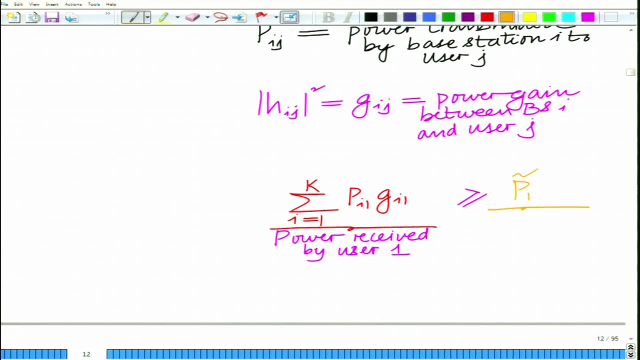 is basically the power received at user 1.. the sum of the powers, correct, that is, the powers, the sum of the powers received from all the base stations. alright, And remember we said this has to be greater than or equal to P 1 tilde, which is the minimum power desired by user 1.. 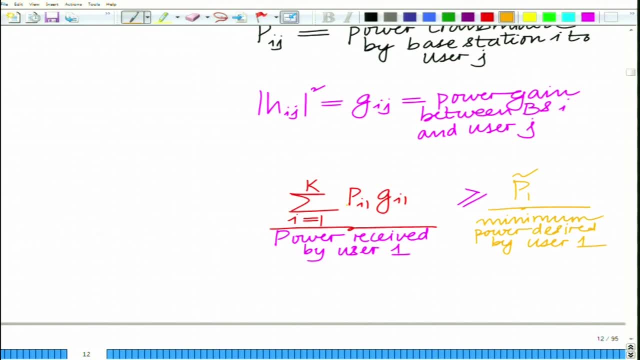 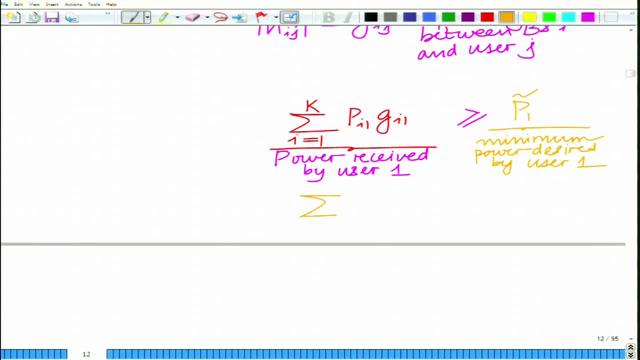 This is the minimum power desired by user 1.. So the sum of the powers received from all base stations has to be greater than equal to P 1 tilde. This has to also hold similarly for the other users. So at user 2 we must have the sum of the powers received from all. 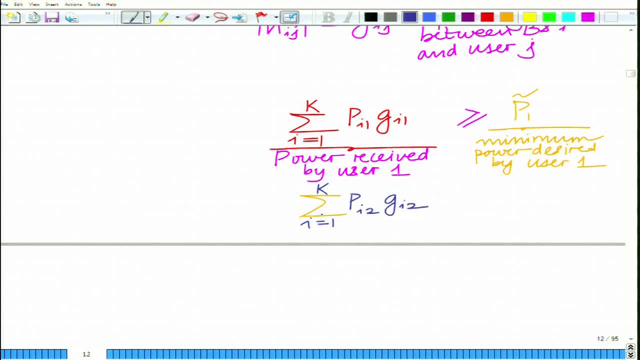 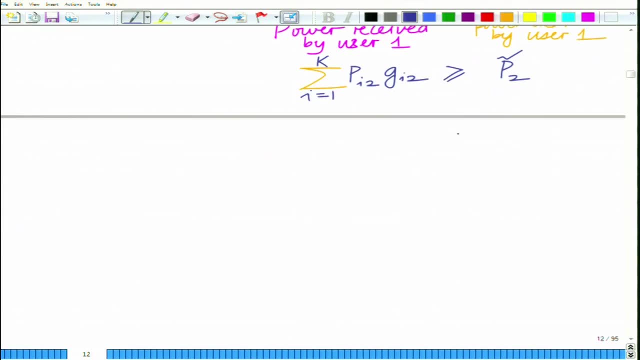 base stations, that is P i 2, G, i 2. summation over i equals 1 to k. over all base stations that has to be greater than or equal to P 2, tilde, and so on and so forth. that is summation i equal to 1 to k. P i m at user m summation i equal to 1 to k. P i m, G i m greater than. 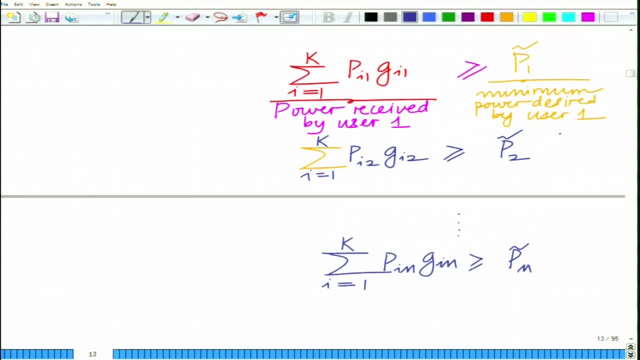 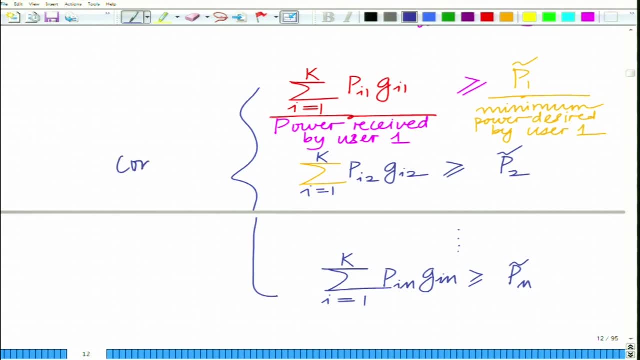 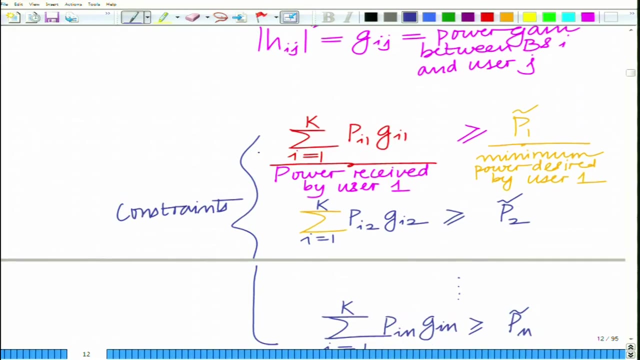 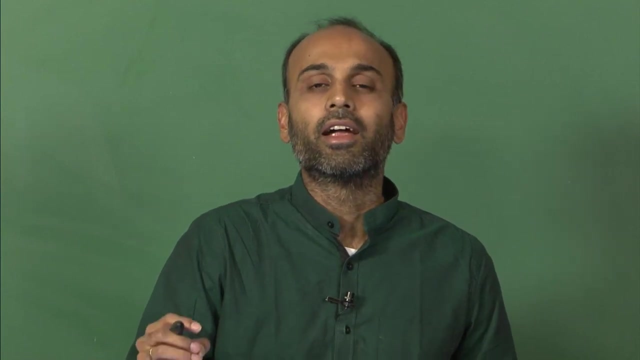 or equal to P m tilde. So these are your constraints and you can see these are basically affine constraints And now we need an objective. one of the objective that one can consider is basically: you want to meet the desired power level at each user. 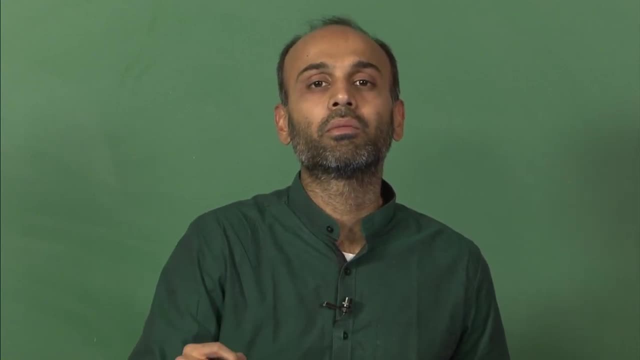 but simultaneously we also want to transmit the minimum amount of power. So what is the total? what is the minimum total power that can be transmitted by all base stations to all users to meet these desired criteria at the various users. So the objective function. 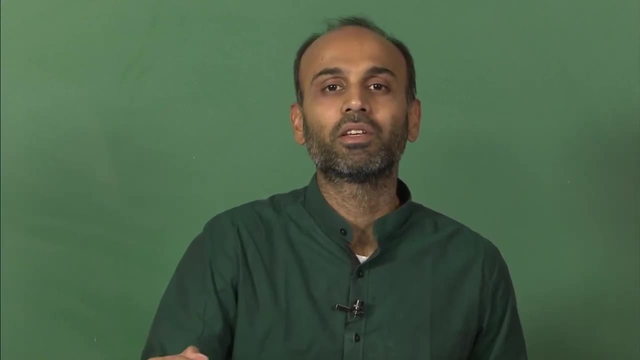 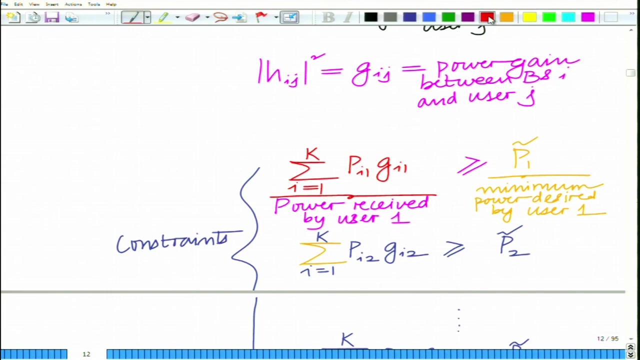 can be to minimize the total power transmitted by all the base stations to all the users. So now that makes it a convex optimization problem. So the objective function can be: minimize summation i equal to 1 to k, summation j equal to 1 to k, summation over all base. 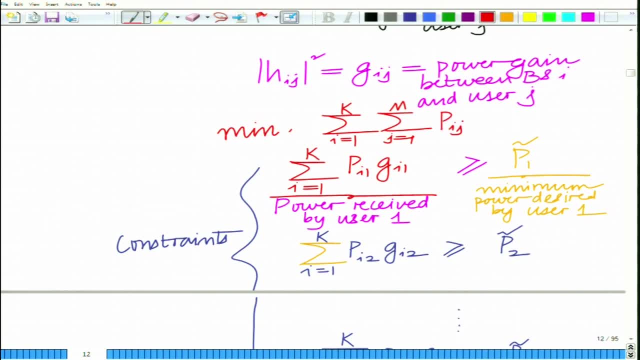 stations. summation over all users: P, i, j, that is, power transmitted by the base stations to all. So this is your linear objective. remember it is simply the sum. So therefore, it is a linear objective, linear objective and this represents- remember, this is the total power by all base stations to all users. 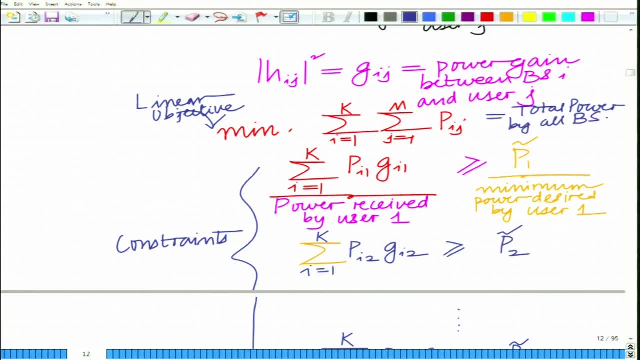 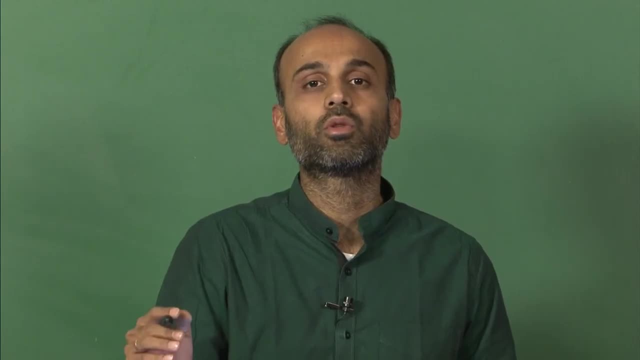 This is the total power by all base stations to all users. So what is our optimization problem? Our optimization problem is to minimize the total power, transmit power of all the base stations to all the users subject to these constraints. That is the mean that 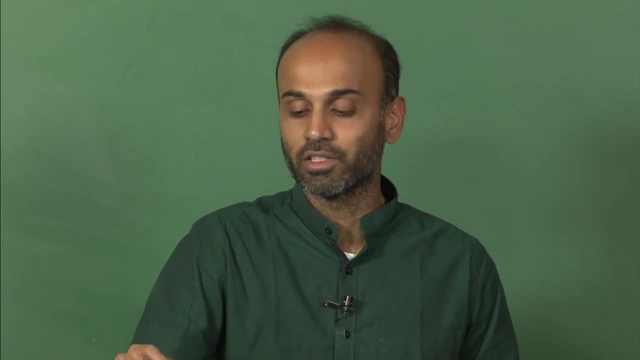 is the power received at each user is greater than a minimum threshold which is denoted by p j tilde. At user 1, it is p 1 tilde. user 2, p 2 tilde, so on. At user m, it is: 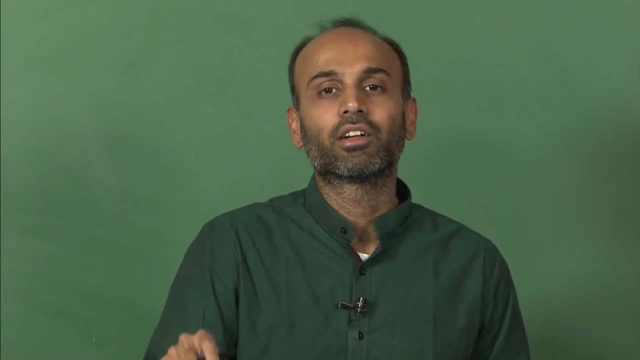 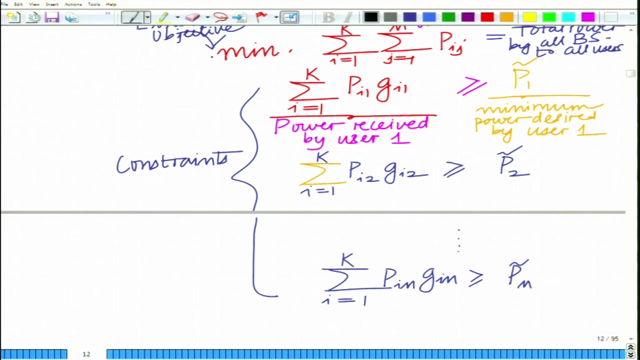 p m tilde, and you can clearly see the objective is linear, constraints are linear, this is a linear program. So this is so cooperative, base station transmission or base station cooperation. this is basically. this is a. one can formulate a base linear program and 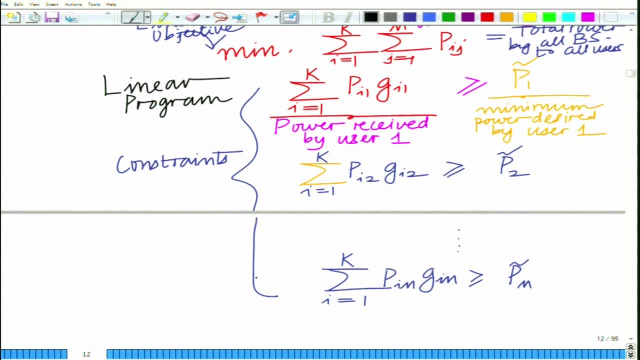 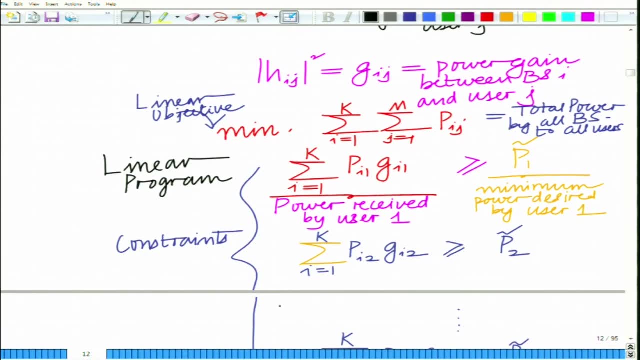 you can see this, the variety, or the interesting and very interesting applications of the simple yet very flexible and powerful optimization framework of that of a linear program. So this can be obtained to minimize the total transmit power, total power that has to be transmitted by all the base stations to all the users. Now also note that in the standard 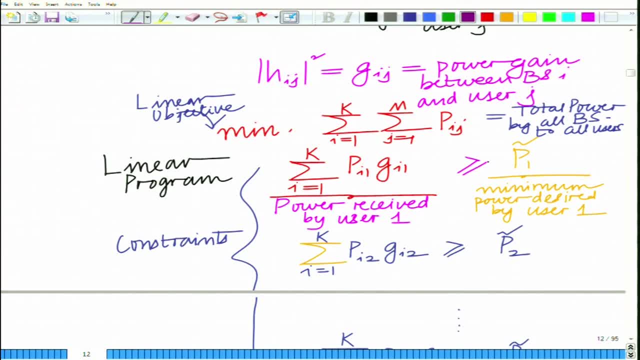 form: convex optimization problem. the inequalities are have to be less than or equal to So, and one can readily convert it to the standard form by simply introducing a minus sign. So I will have a minus in front of everything, and if youguru over the next straight line. this is the number of advantages. this will be l minus l minus i, equal to alpha function. if I think dramatically, you will be able to desperate the exact orders of each condition and fit it in a solutions. So that is an extreme scenario. fiveża range of problems which we are now going to learn here. As I said, the linear linear, and it will have particularpelled optimizations, which requires major regularization or linear program scenarios, which is again an absolute. 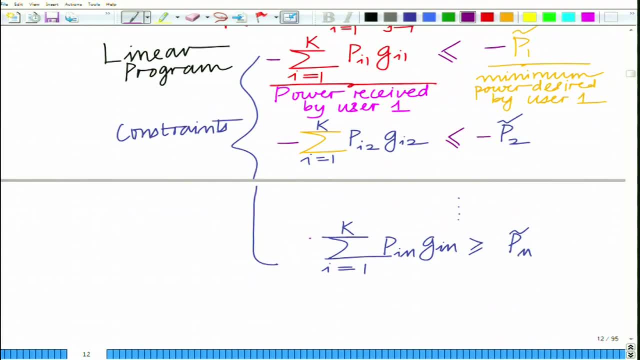 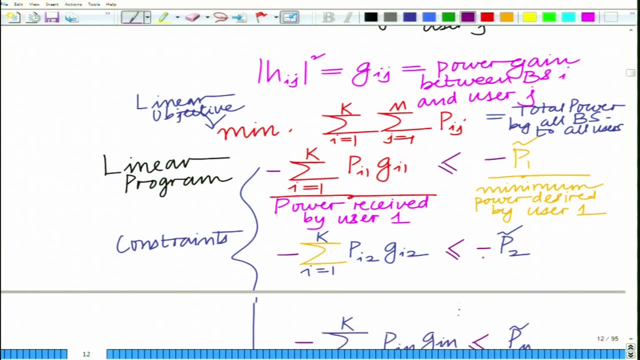 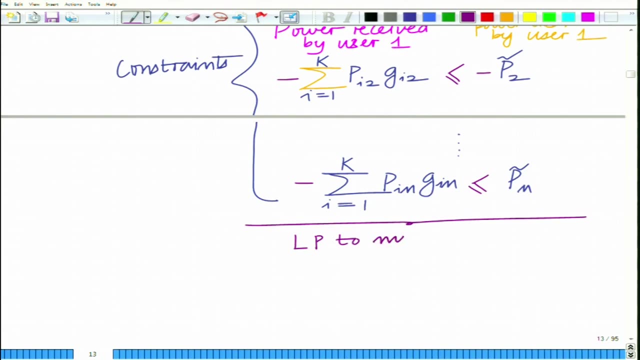 and the inequalities become less than or equal to. So this becomes: minus is less than or equal to, and this is now your standard form, linear program. So this is your L? p: to simply minimize total transmit power of base stations to all the users. 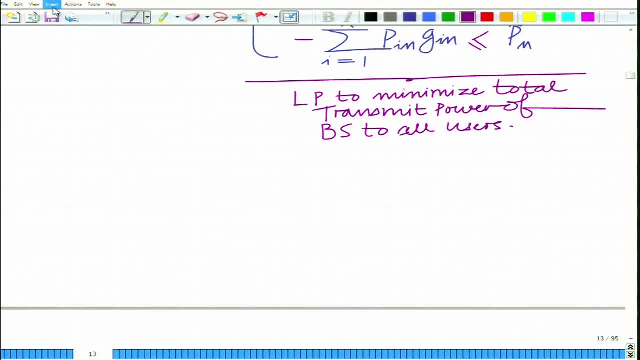 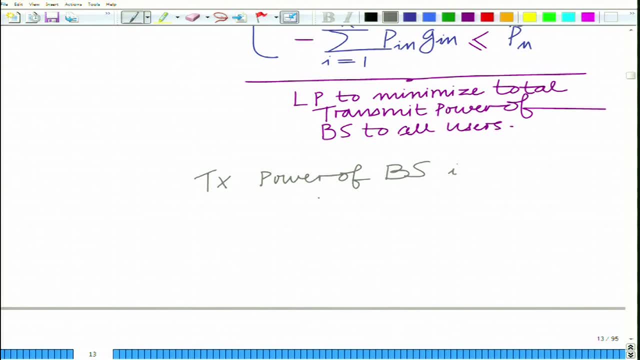 base station i, that will be equal. that can be represented as p of i. So the transmit power of base station i can be represented as p of p. i equals summation, that is, the power transmitted to all the users, summation over all users. 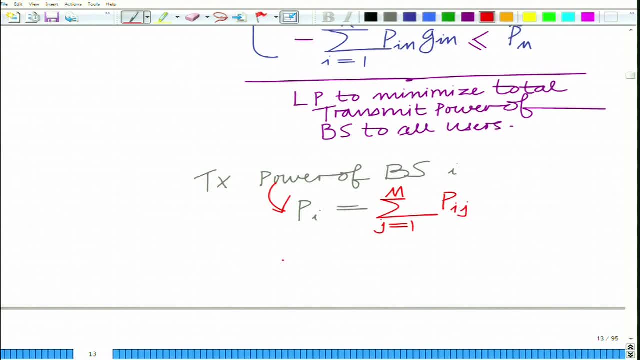 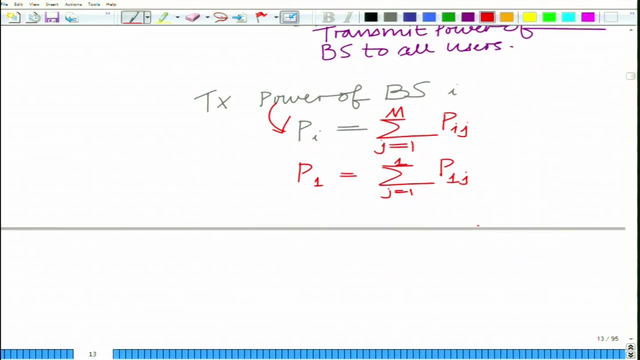 So this is power transmitted by base station i equals to j. equals to one to m, p i or p 1 j. that is the power transmitted base station i to each user, j summed over all the users. So this is power transmitted by total transmit power: M i over p 1 of j. So this p i will. 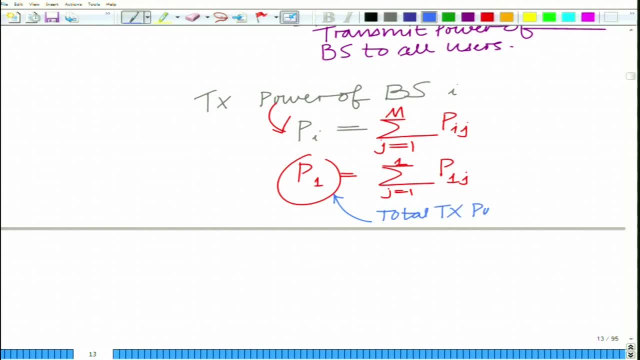 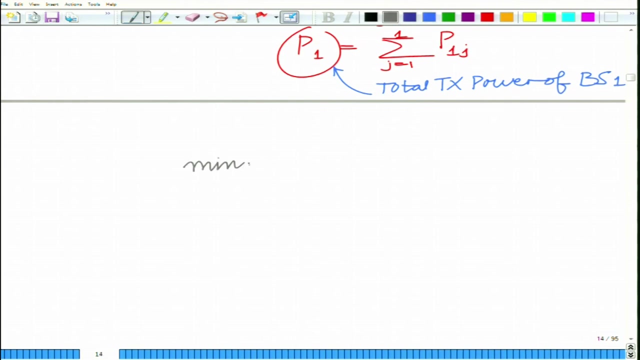 be equal to m p i over p 1 of j. So this power transmitted by base station i. So this power of base station 1 in fact, that is what this is. And now what we want to do is we want to consider interesting optimization objective function in which we want to minimize. 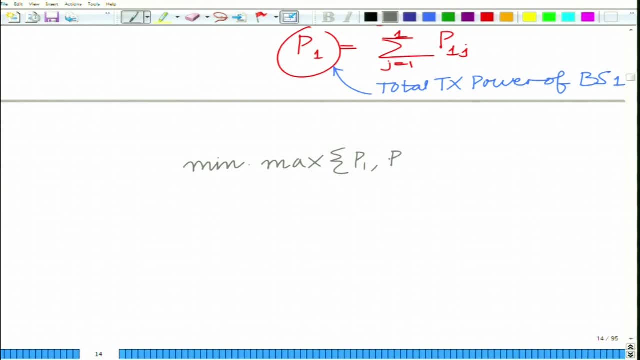 the maximum of the powers transmitted by the various base stations, So the total K base stations. so you have transmit powers V K. So you want to minimize the maximum. so what this is doing is minimizing the maximum power transmitted. So 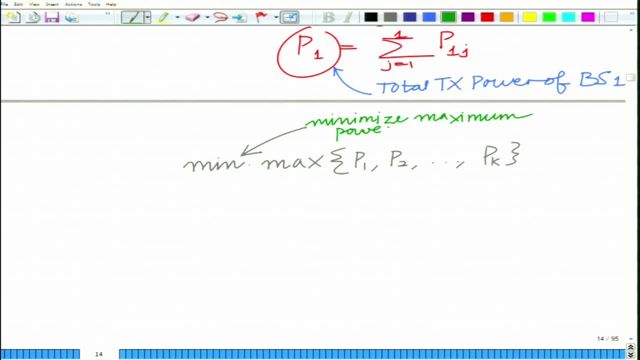 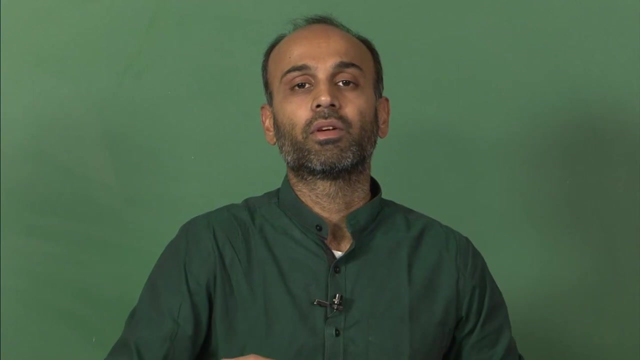 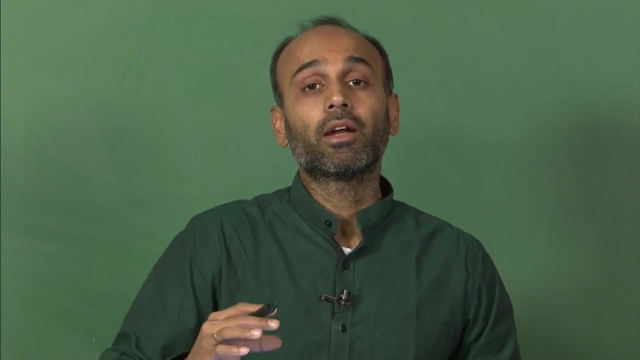 transmitted, minimize the maximum power transmitted by base station. Now, what happens typically in this cooperative cellular scenario is that there are few base stations. there are few. there are several base stations, and what? when you minimize the total power transmitted by all the base stations together, that might result in an undue burden. 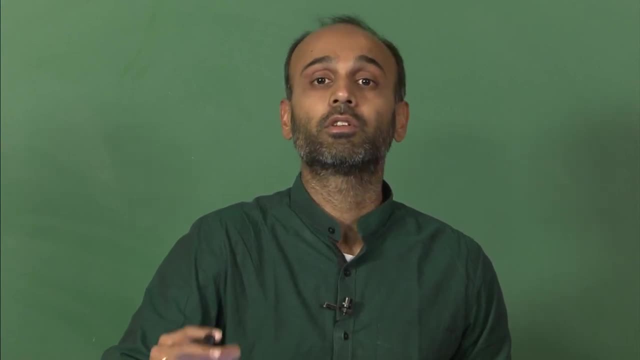 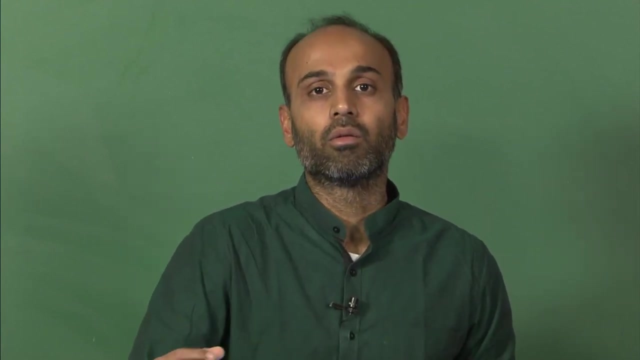 on a single base station. So one of the one particular base station which probably has good condition- good channel conditions of where the channels to the different users are good- can be overburdened or overtaxed in comparison to. So this does not ensure that the load is so the previous total power minimization does. 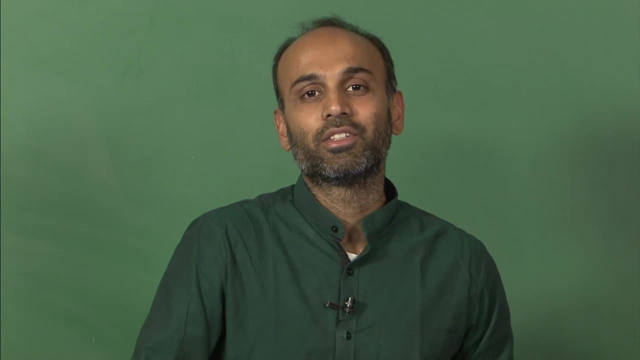 not ensure that the power is uniform, that the power load, that is, the burden, The transmit power burden, is not uniformly levied on all the base stations. there might be different base stations which are which are levied more or which have to transmit. 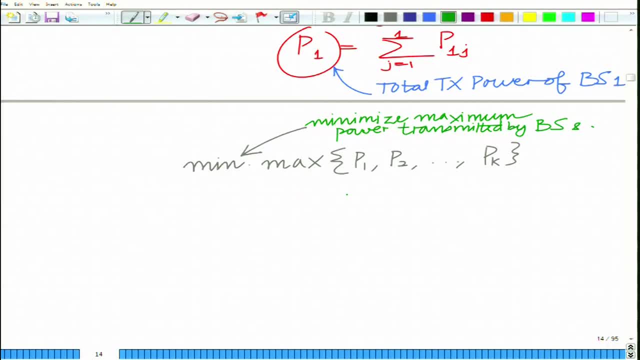 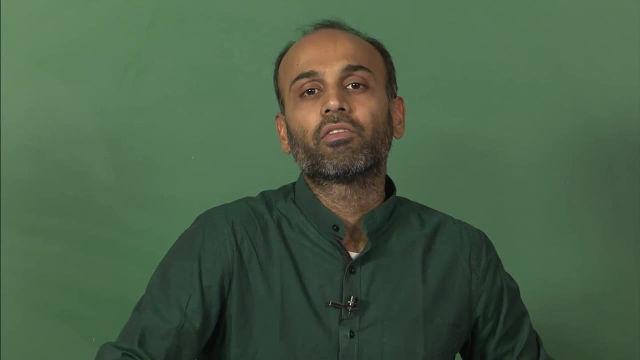 more power in comparison to others, But when you are minimizing the maximum transmit power, what this does is that this ensures a sort of fairness in the power burden. it sort of ensures that this power burden for the different users is rather uniformly, rather fairly distributed on all the base stations. 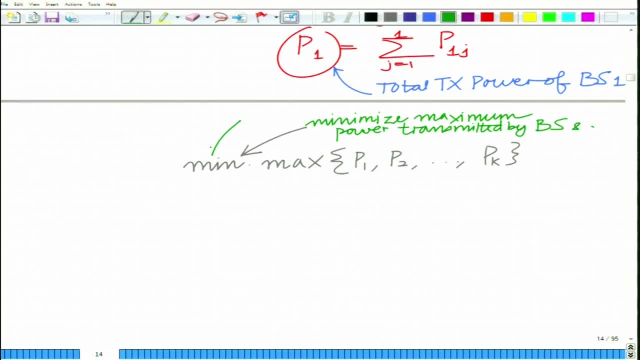 So this is an important property of such problem. So this ensures you can say minimax. the minimax criterion basically ensures fairness in the power burden, in the power power burden or the power distribution, minimizes the maximum power And, subject to the constraints, are all are there, as usual. that is, if you look at the 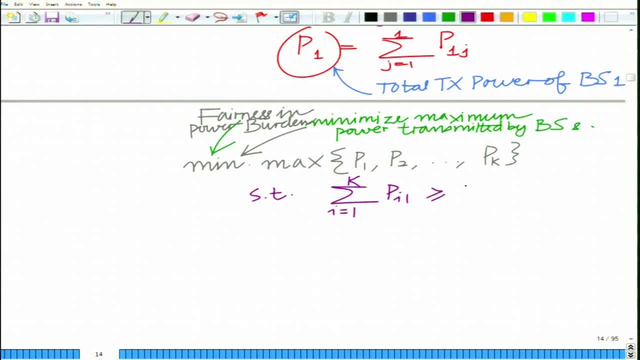 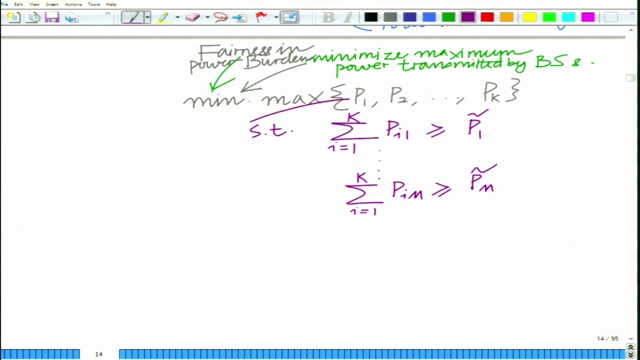 desired power At each user that has to be greater than the threshold. so the constraints are there. so this is Now, if you look at this minimax now, if you look at now, if you look at each P, i and 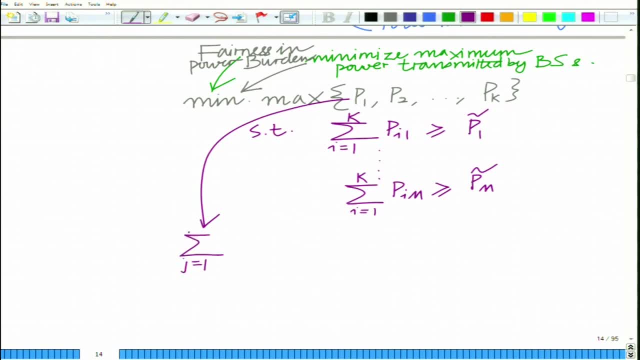 we already seen this. each P i is summation j equals 1 to m. Ok, This summation j equals 1 to m. P, P 1, j and this you can see, this is affine, or this is convex. So each of these P 1, P 2, P k, each of these powers, 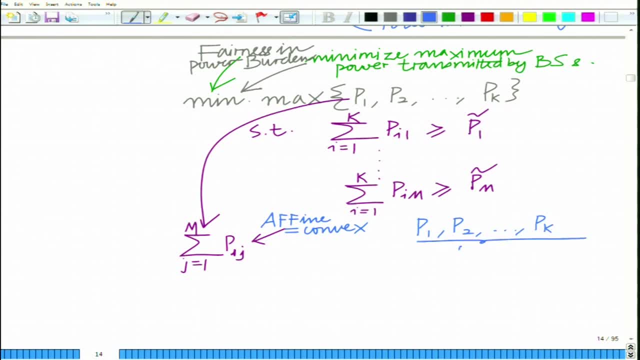 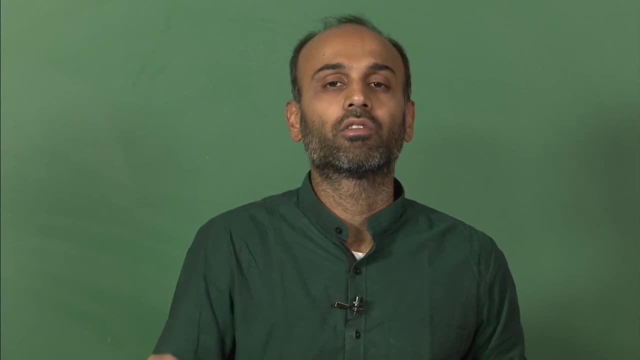 So each of these is convex and therefore, when you take the maximum of this, remember the maximum of a set of finite or infinite convex function is convex, All right, And therefore the maximum of this set is convex. So this implies: 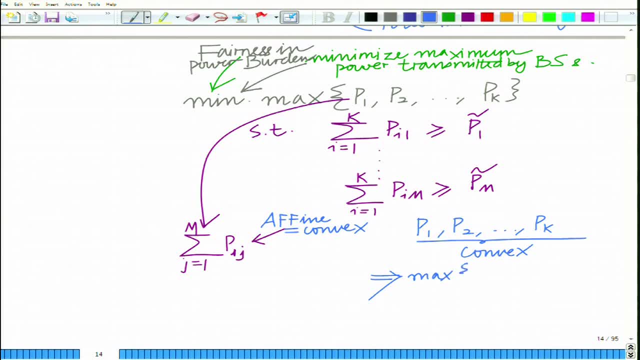 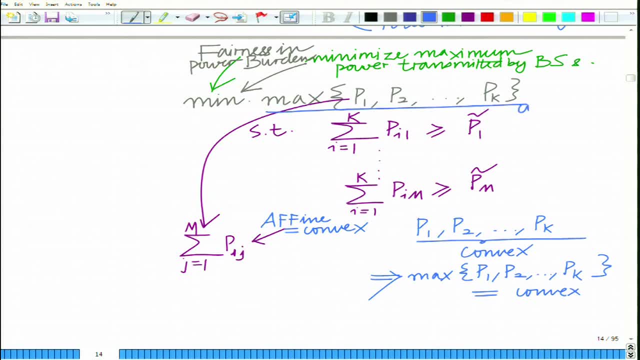 Constraints are as usual, I mean similar to the previous one, When they were convex. So this is also a convex define function. So this 시간 is also called as convex конечно. So it implies it means that this time it isamelos to left side, and also it implies 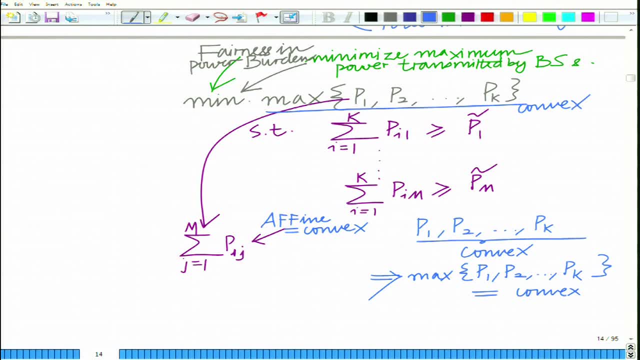 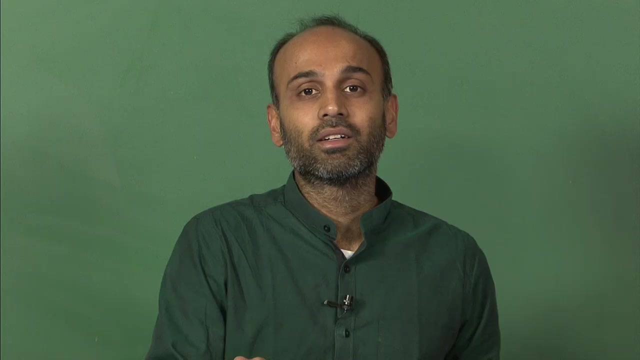 convex objective function. Ok, OK, Ok, Ok, Ok. So these parameters have also been explained. Ok, convex optimization problem, And this is also, therefore, convex optimization problem. Now, what is its relation to a linear program? Now, at present, it seems unrelated to a linear. 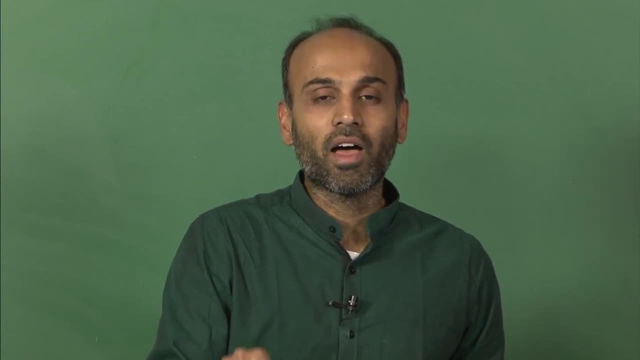 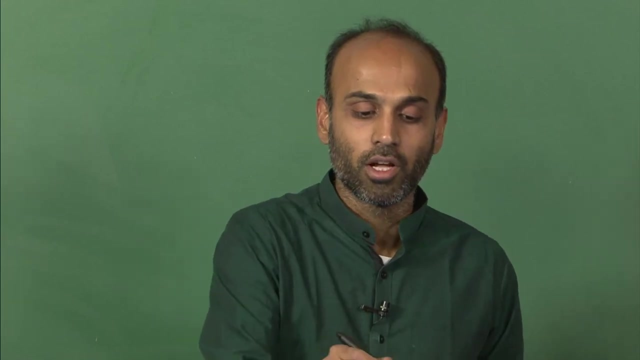 program, but we are going to demonstrate that this is in is in fact can be written as an equivalent linear program, And for that we will use the epigraph trick that we have seen in the previous module. So how can this be written as a linear program? So we have minimize. 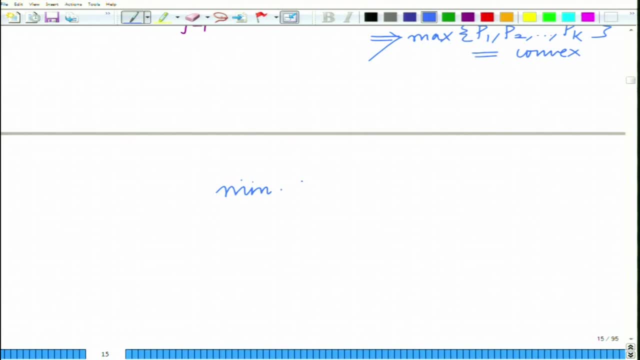 now we will use the epigraph form, So I can write this as: minimize t, subject to the objective maximum of p 1, p 2, p k. This is less than equal to t And the rest of the constraints are as usual there, that 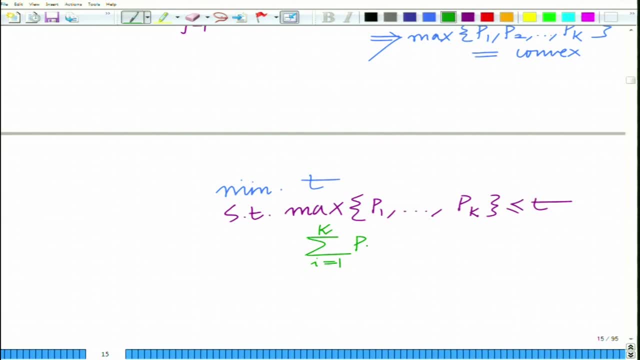 is summation i equal to 1 to k. p i 1 greater than or equal to p, 1 tilde, and so on and so forth. Summation i equal to 1 to k and k 1.. So this is less than or equal to t And I. 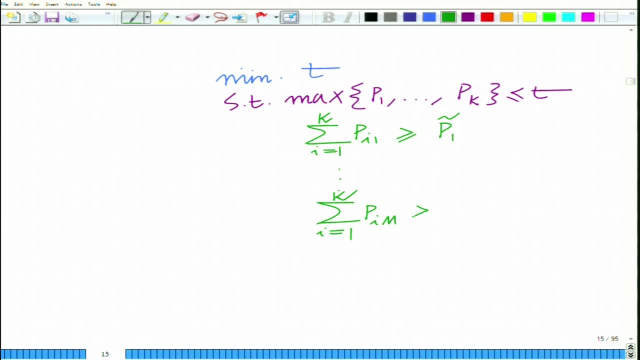 P i m greater than or equal to P m. tilde Now the maximum of P 1, P 2 up to P k less than or equal to T. the maximum of a set of quantity is less than or equal to T if and: 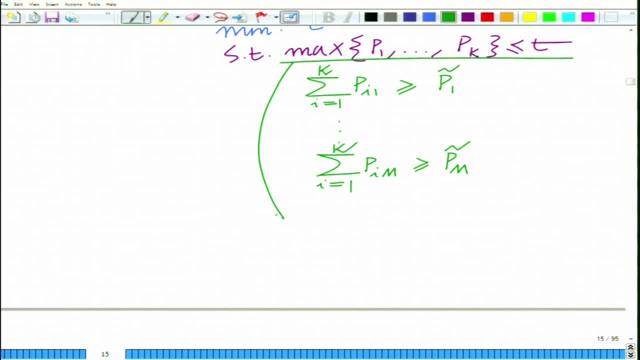 only if each of these is less than or equal to T. So this implies each is less to be each P. this implies each P i has to be less than or equal to T. And now I can write the equivalent optimization problem. Therefore, this is optimization problem is equivalent. 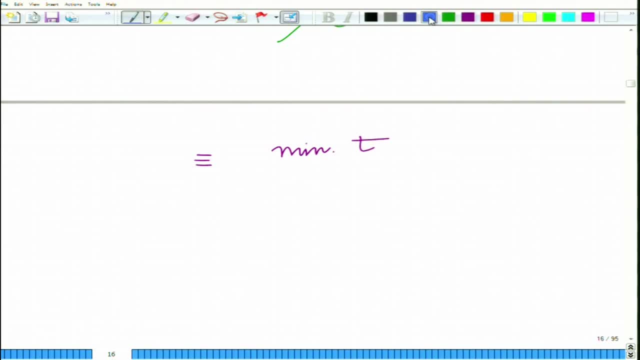 to minimize T subject to now, we need that each P i is less than or equal to T. So this means P 1 equals summation. j equals 1 to m. P 1: j less than or equal to T, j equals 1. 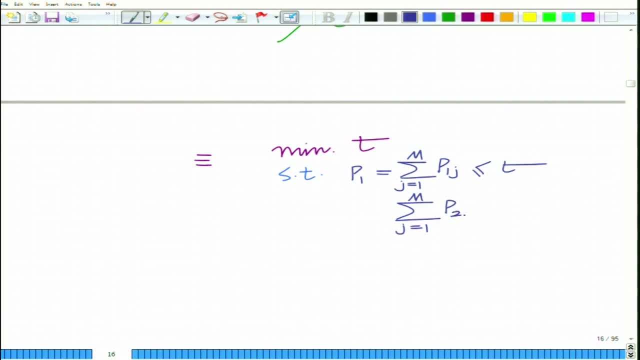 to m P 2 j. summation less than or equal to T. This is the power transmitted by base K, base station 2 to all users. and finally, summation: j equals 1 to m p k. j less than equal to t. 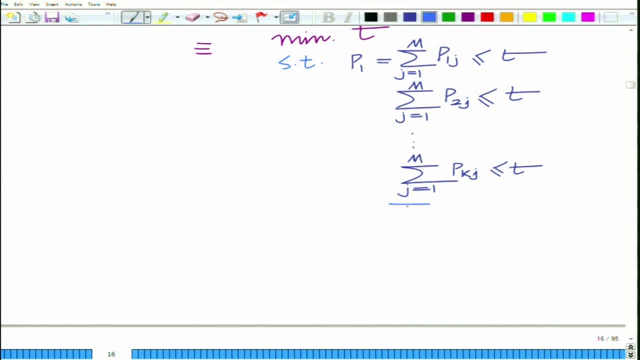 These are the base station power constraints and you have the user constraints as well, similar to previous. So summation i equal to 1 to k. p i is equal to i. 1 greater than equal to p. 1. tilde summation i equal to 1 to k. p i m greater than equal. 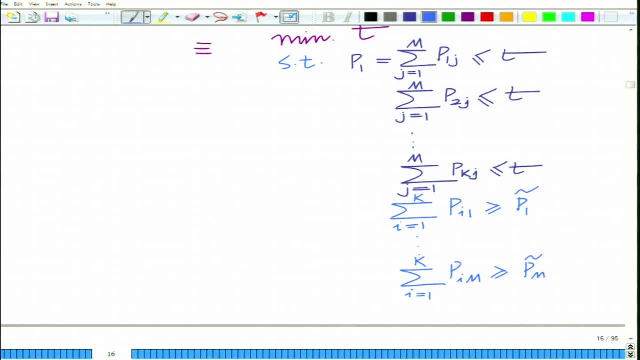 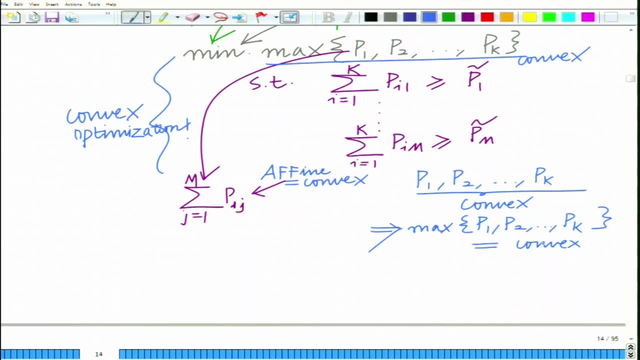 to p m tilde. I am sorry this has to be. I am missing. I am missing here, missing the channel gains. the channel gains are very much there, So this has to be g i 1 g i m greater than equal to p 1 tilde, p m tilde and similarly. 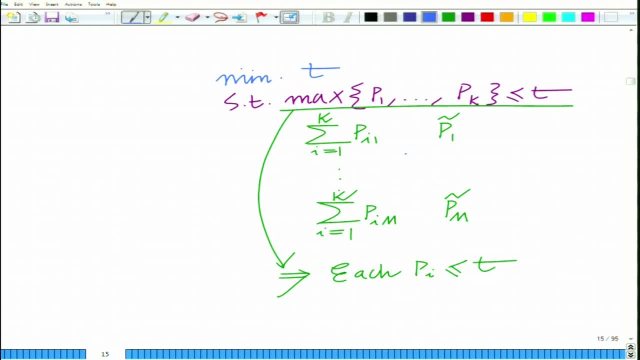 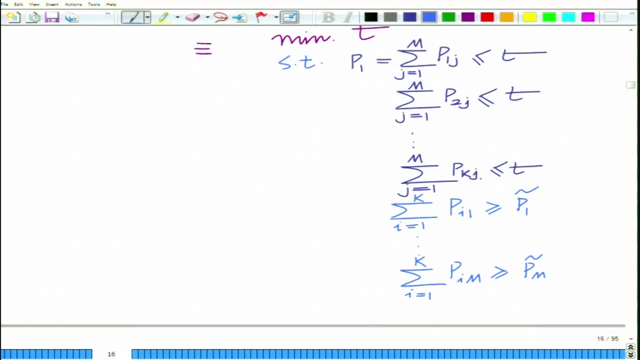 this has to be p i 1, g i, 1.. So on the fourth summation, p i m, g i m greater than equal to p m tilde. Similarly, here also summation i, equal to 1 to k. p i m, g i m greater than equal to p. 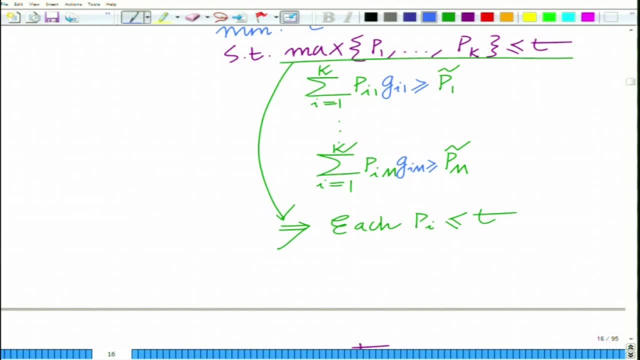 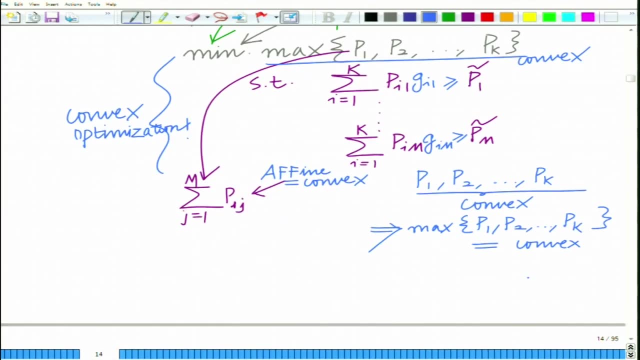 m tilde, Just let me make sure that we are not missing this at any point. Yes, in fact, I think that. so that, Yes, so we want to minimize, Okay, The maximum Correct. Using the epic graph form, I can write this as: minimize t such: 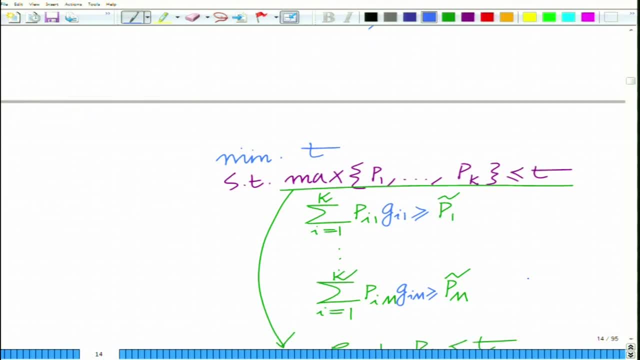 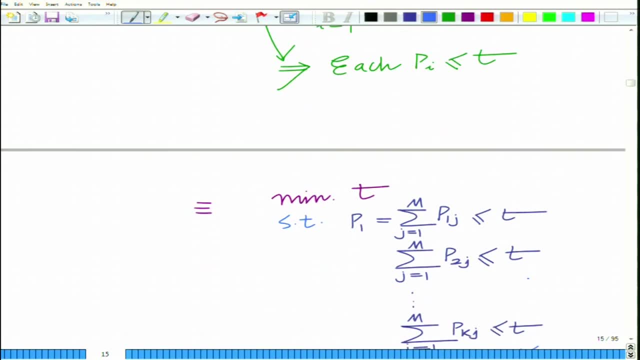 that the maximum is less than equal to t. The desired power at each user has to be greater than or equal to p j tilde. That is there, as usual, and if the maximum is less than T, then we have each p i is less than T, which implies that 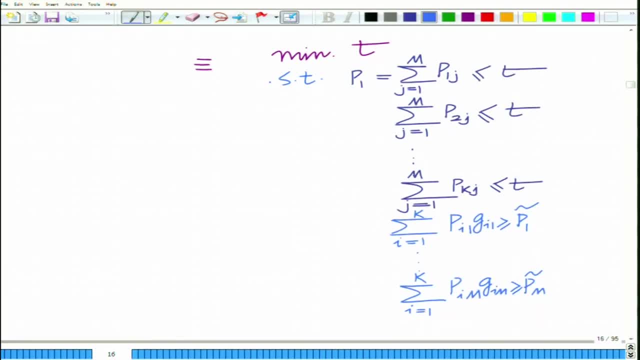 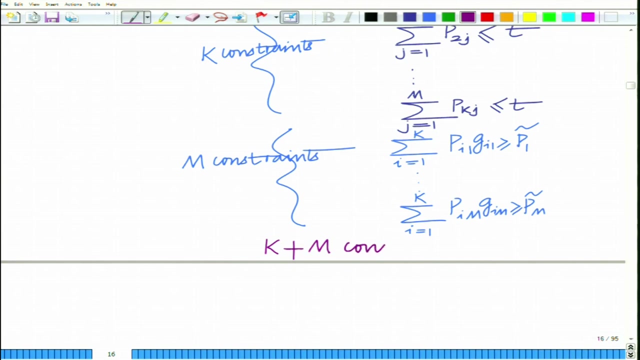 that, So I can write this as so. now we have. this is basically the K constraints and you can see each is an affine constraint and this are your previous M constraints. So the Minimax optimization problem has K. this has a total of K plus M constraints, So this has a total. 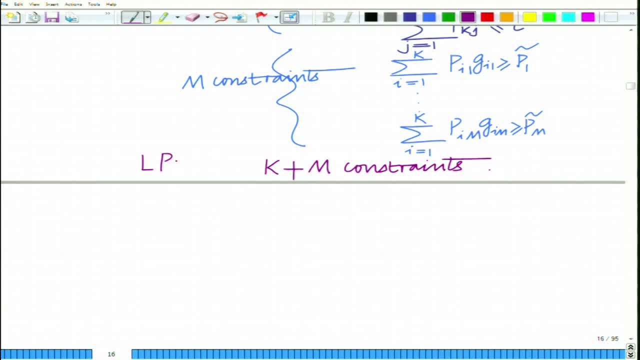 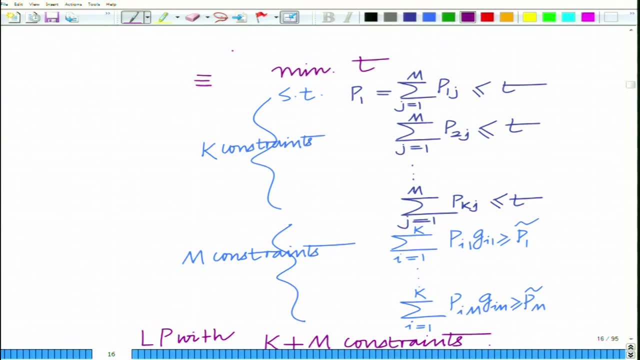 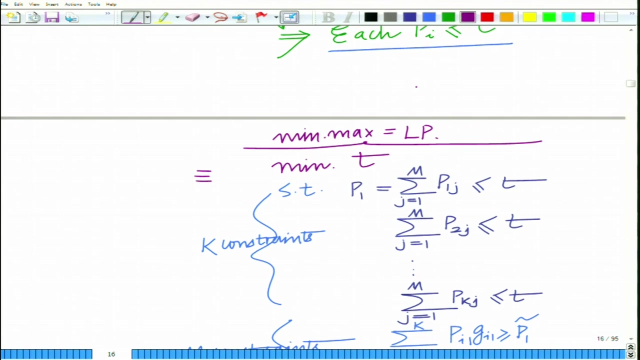 of. so this is a, so you can write the Minimax. So this is also an L P, So you can see each of these. all these constraints are affine. So therefore, the Minimax problem, this is also a linear program and it is not obvious in the first instance, but using a clever 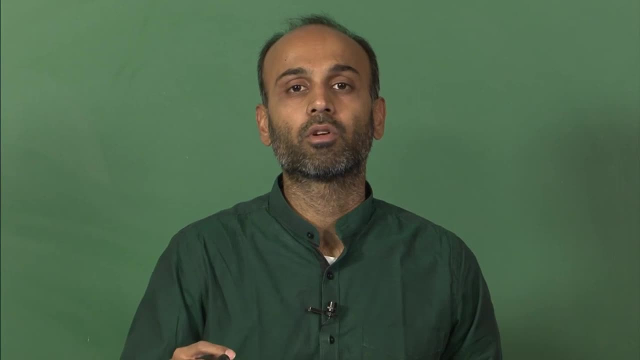 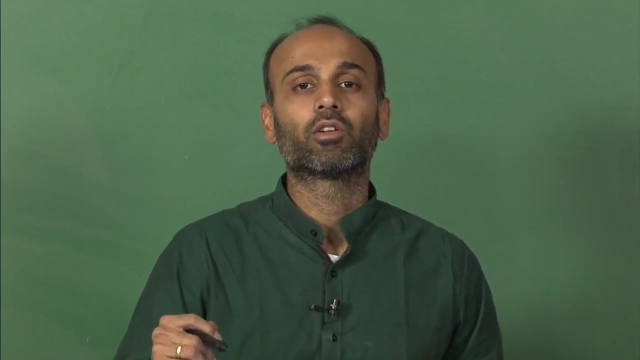 trick, all right, or by manipulating this, you can write the Minimax problem as an equivalent linear program and therefore the linear program has can be written in various forms and has very interesting application. So not only can be used to minimize the total transmit power, but you can also be used to, as I have said, it also. it can also be used 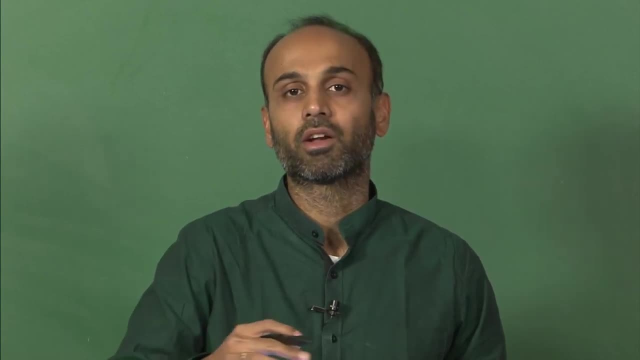 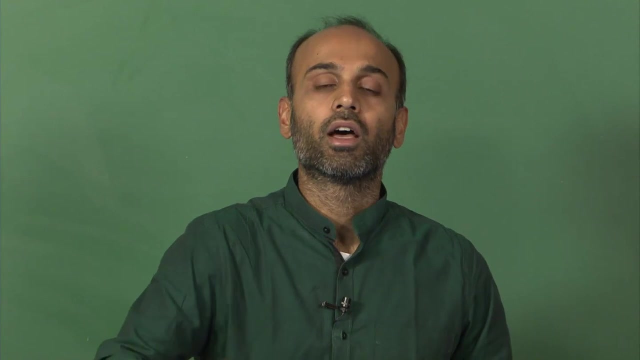 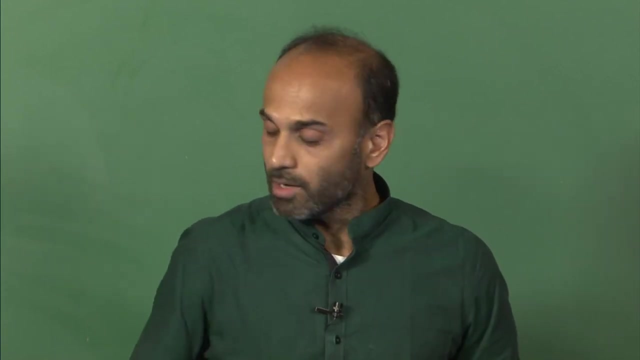 to minimize the maximum Maximum transmit power, maximum power transmitted by any base, any of these base stations, thereby ensuring that this power burden, or the transmit power burden, is fairly, or it is sort of evenly, distributed on all the cooperating base stations. all right, So that basically introduces the 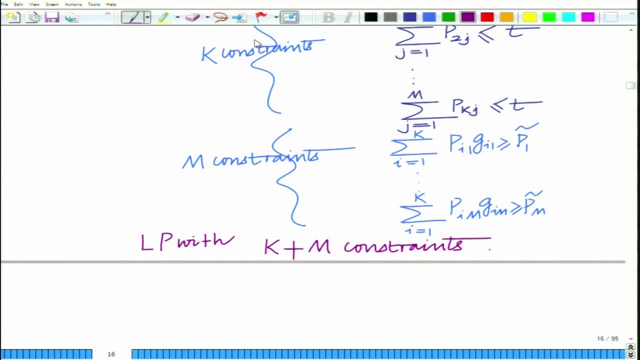 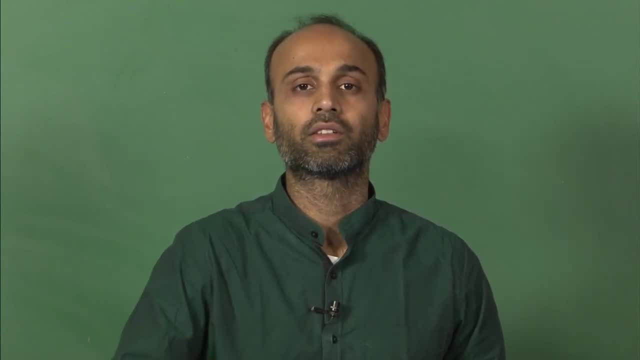 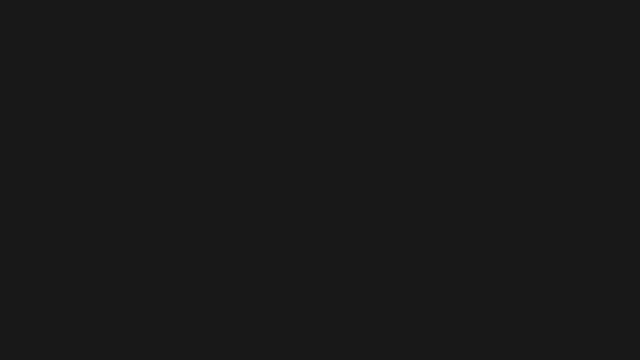 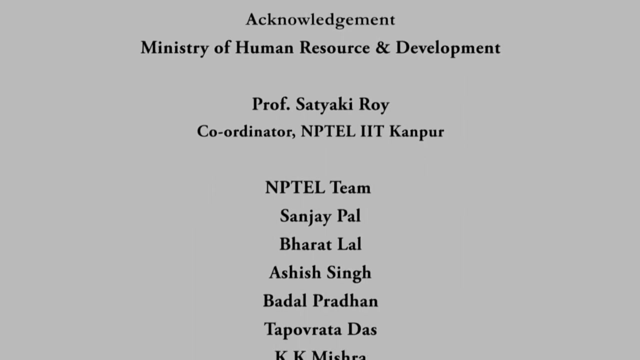 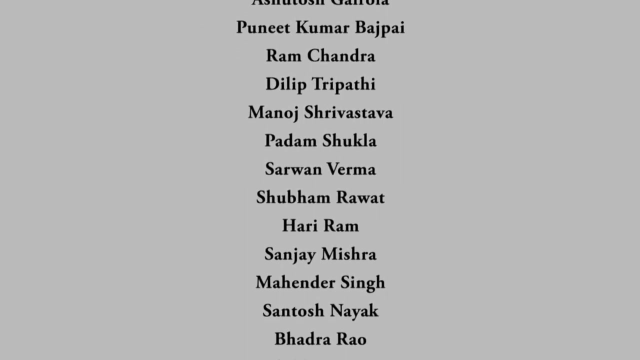 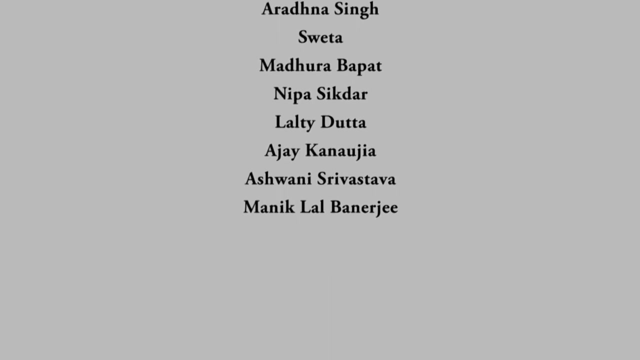 linear program and basically demonstrates its application in a practical, in a practical wireless scenario. So we will stop here and continue in the subsequent modules. Thank you very much, Thank you very much.